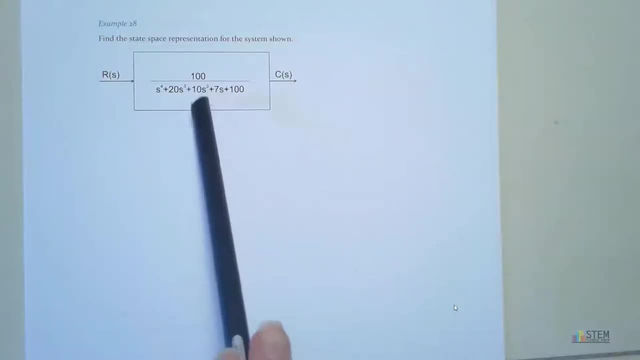 Hey guys, what we have here is a transfer function right here, That's G of S. We've got R of S as our input, C of S as the output, And what we want to do is we want to convert this transfer function over to state space. Alright, that's what we're going to do Now. 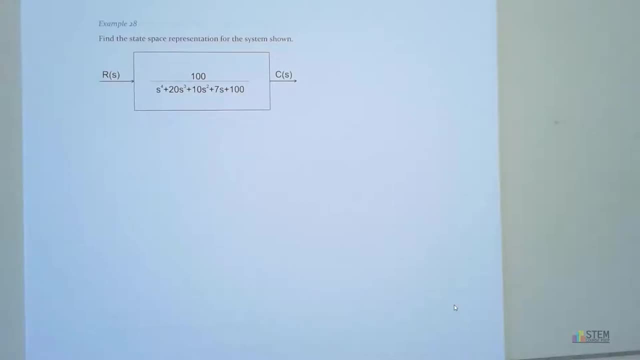 if you remember, in that last video when we covered the theory behind this, I didn't show you how to actually go from the transfer function to the differential equation, So we're going to do that in this example. That's easier to just show you with an example. so 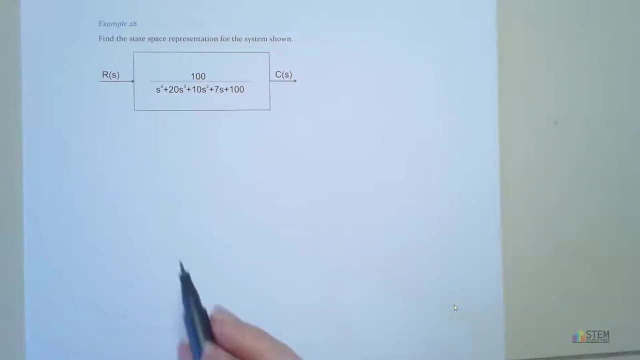 I figured we'd do it here. Alright, so what we have here is this transfer function. Remember, a transfer function is output over input. So that means we have C of S over R of S And we're going to set that equal to this transfer function. So we have 100,. 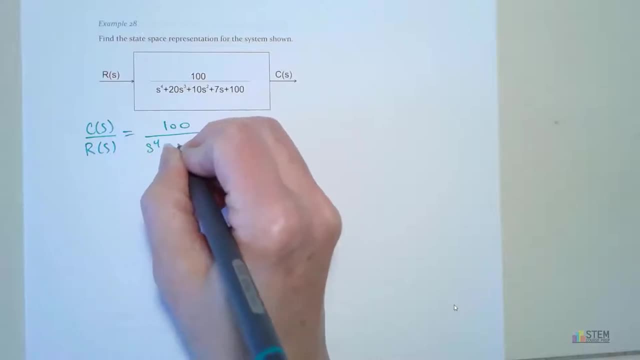 put that over S to the 4th, plus 20S cubed, plus 10S squared, plus 7S plus 100.. Now we've got that. Now we're going to use this to get our differential equation, What we're going. 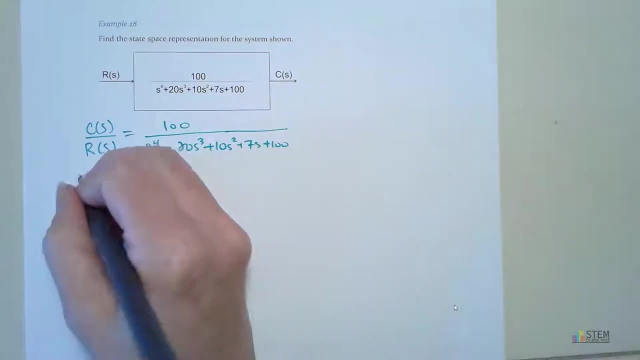 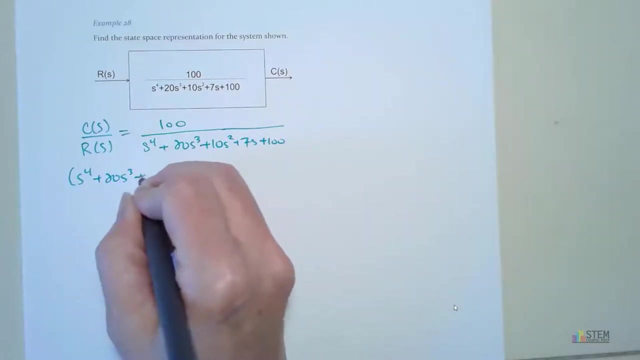 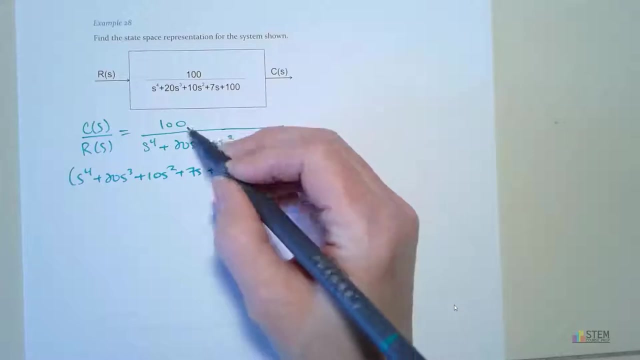 to do basically is cross multiply. So we have this denominator, we're going to multiply it by C of S. So we have that, put it by C of S, and then, right side, we're going to have 100 times R of S. Like that, Easy enough, Okay. so now we've got this equation. This is essentially. 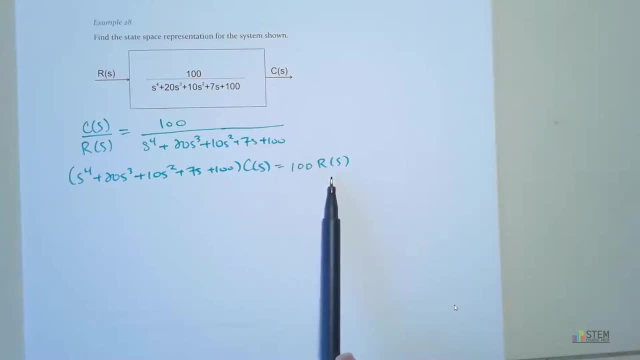 the Laplace transform of your equation of motion. Now what we're going to do is basically just do the inverse Laplace of all of these terms. We're going to assume initial conditions are 0. So let's put need differential equation. So let's take the inverse Laplace And this: 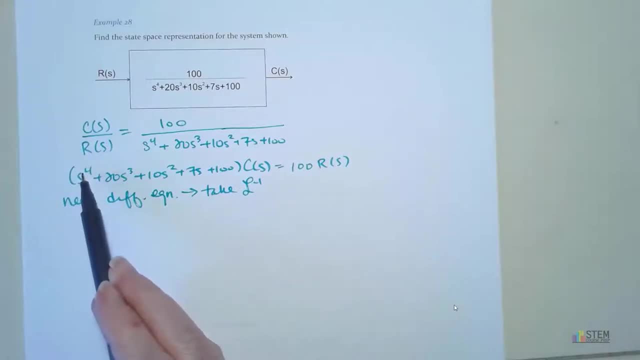 is easy to do. The exponent on S tells you the order of the derivative. Alright, so this is S to the 4th times C of S. So that means we've got the 4th. I'm just going to put a. 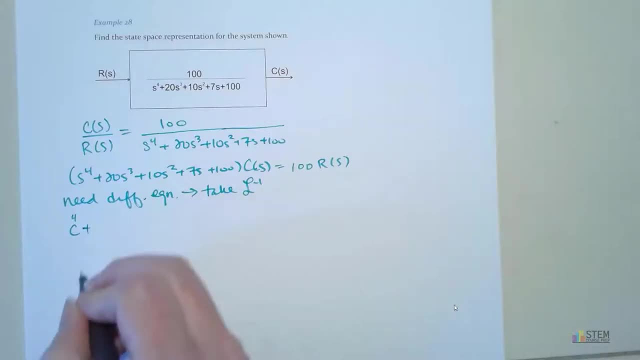 4 here, the 4th derivative of C, And then we're going to have plus, And then we're going to have plus, And then we're going to have plus. We've got 20 times S cubed, times C of S. So this is cubed, so that means that's the 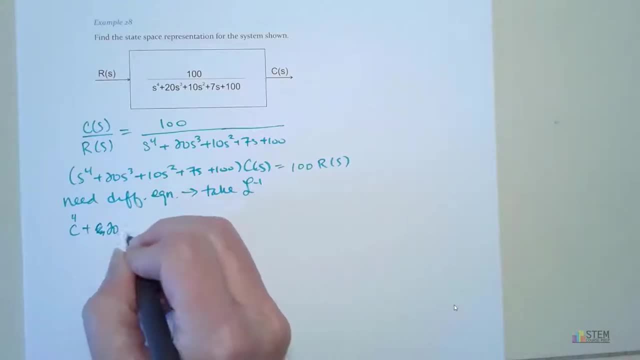 3rd derivative of C. I've got to put 20 in here, So we're going to have 20 times the 3rd derivative of C. And then next we've got 10 S squared C of S. This squared indicates 2nd derivative. 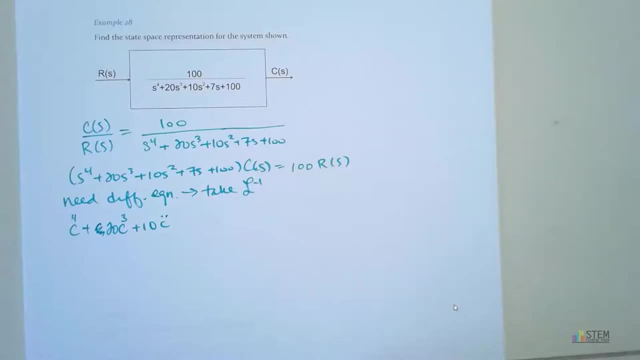 So we'll have plus 10 C double dot. Then you just keep going. So 7 S, that exponent is 1.. So that means we're going to have 7 times C dot. Finally we have 100 times C of S. That just gives us plus 100 times C And then it equals. 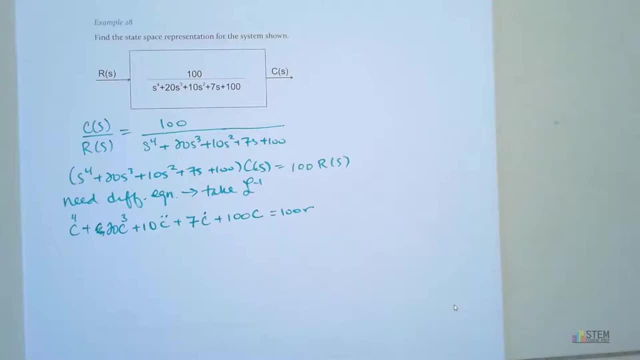 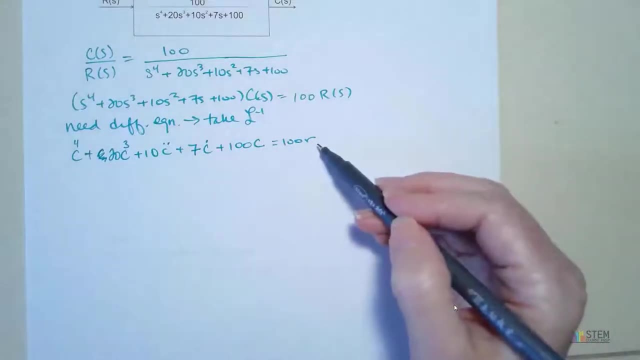 100 times R. Alright, so you just work backwards, And this is kind of what you would do. actually, it's not kind of. it is what you would do if you did the impedance method and you needed to get a differential equation. You would 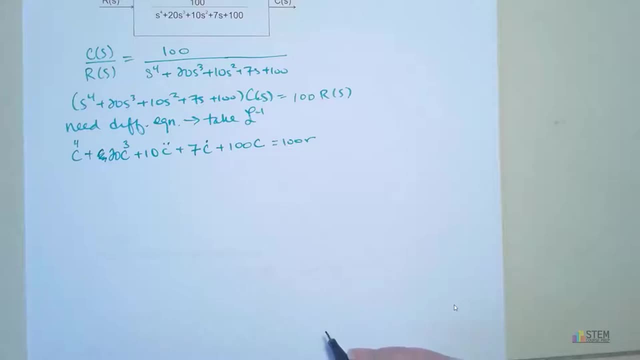 just kind of work backwards. Now we've got this: Our output is going to be C because that's our dependent variable here. So our system variables we're going to have X1 equals C And then we're going to go down. 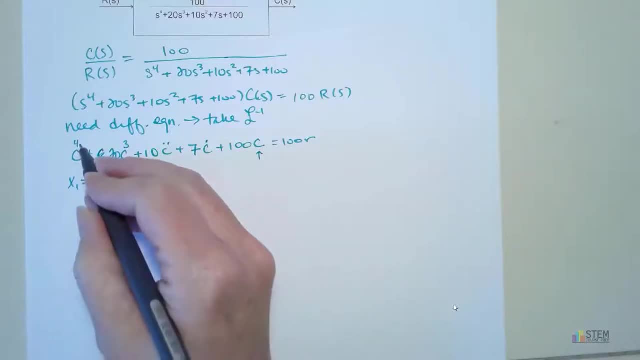 until we get to the N minus 1 derivative. Well, we have C to the 4th here, So that means N is 4.. So we're going to go to the 3rd derivative. Okay, So X2 will be C to the 4th. 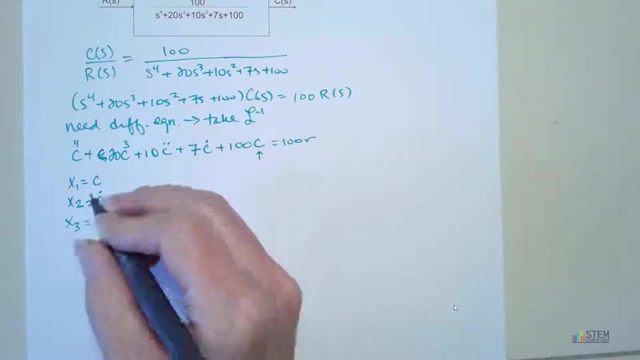 Okay, So C dot, X3 will be C double dot, And then X4, let's put C3 for the 3rd derivative of C. Now take the derivative of all of those: X1 dot gives you C dot, but C dot is X2.. 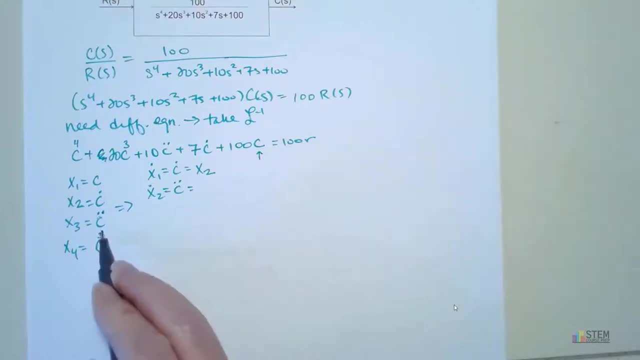 X2 dot is C double dot, but C double dot. C double dot is represented by X3.. X3 dot will be the 3rd derivative of C- Actually let's just leave it the 3 notation- And then that is represented by X4.. 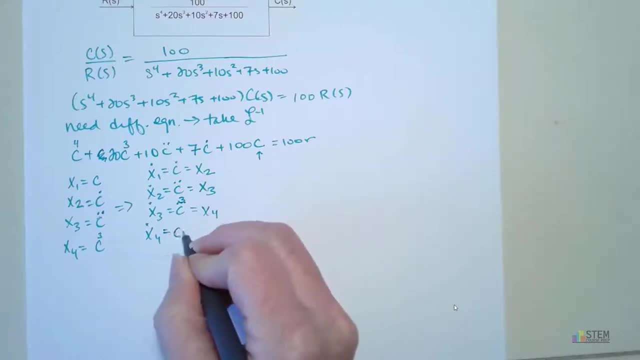 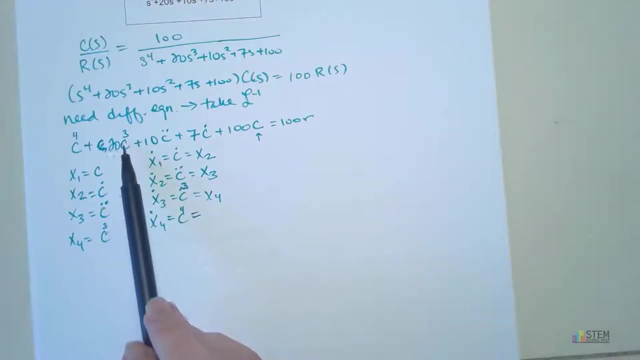 Finally, we get to X4 dot And that's going to give us the 4th derivative of C. All right, so we've got the 4th derivative of C. That's going to take us back up here. We've got to solve for this. 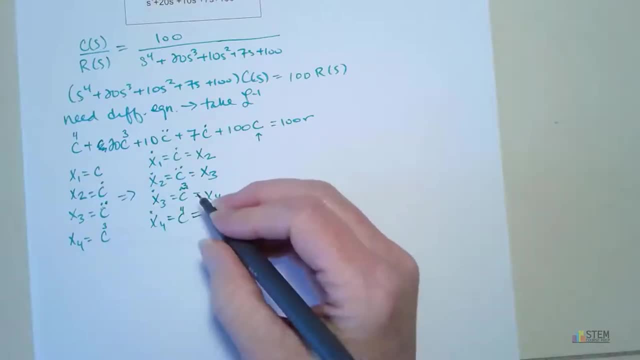 So let's move all this over and that's going to give us negative 20.. We have the 3rd derivative of C, That's represented by X4. Then we're going to have negative 10. We've got C double dot. 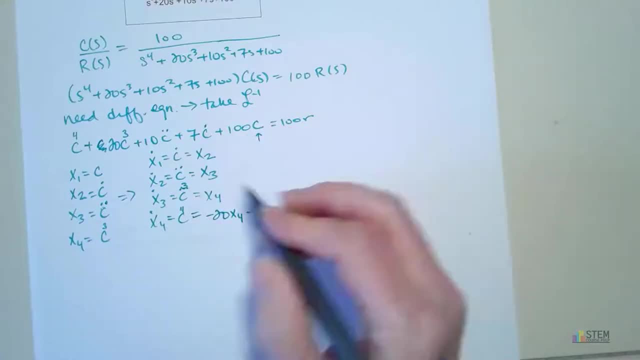 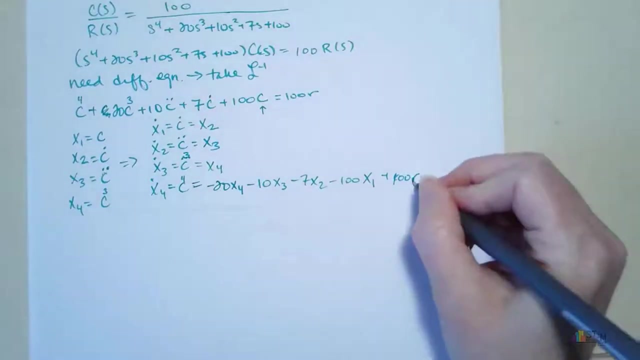 Well, that's X3.. We've got minus 7 C dot, but C dot is X2.. We've got minus 100.. We've got C, but that's X1. And then plus 100. 100 R- OK. so now we have that, we're ready to do the matrix form. 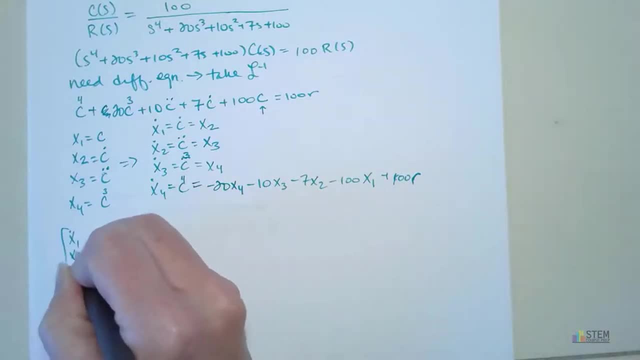 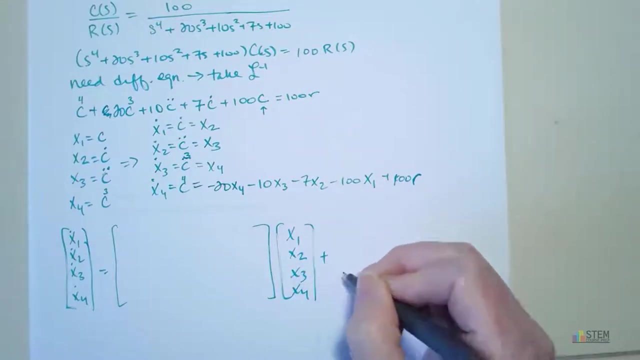 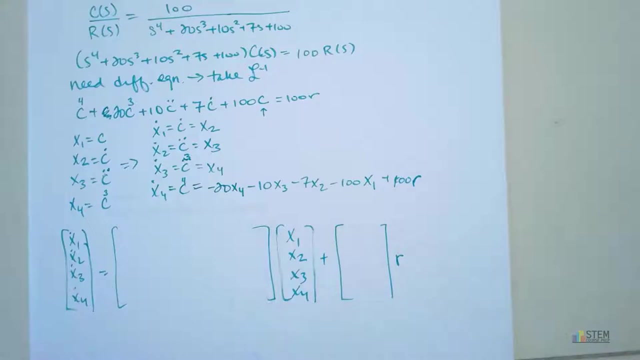 So the derivative of your state vector goes on the left, And then we get our matrix A, Got the state vector, And then plus matrix B times R, Which is our input, And now you just have to fill in the coefficients. So remember, you're going to have that diagonal of 1's until we get to that last row. 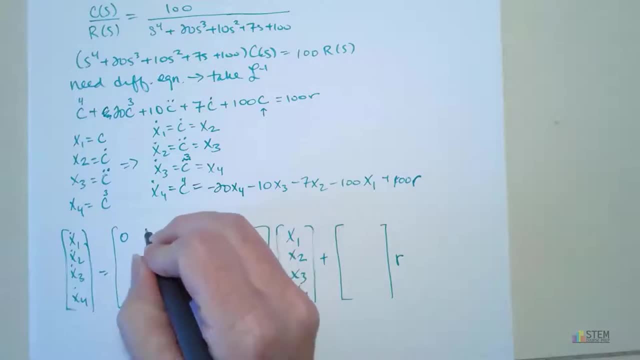 So notice, we're starting out at X2, though, so you're going to have a 0 here first, And then 1, 0, 0.. This over here is going to be 0, because there is no R component in that equation. 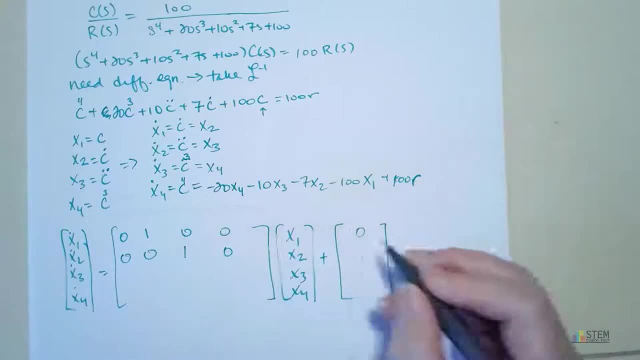 Next we've got X3.. So that's 0, 0, 1, 0.. Over here is 0.. Third row, three 0's, then the 1, and a 0 in the B matrix. Finally, we pull out all of these coefficients here.